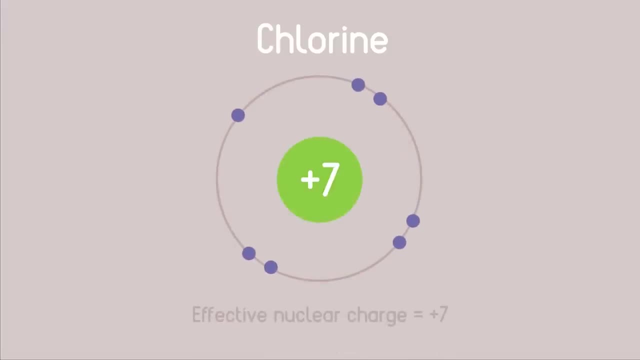 just seven, plus holding them in their outer shell. Sodium with eleven protons and eleven electrons has also ten inner electrons, leaving an effect charge of only plus one to hold its single outer electron. Thus we see why non-metals with nearly full shells hold onto their electrons more strongly. 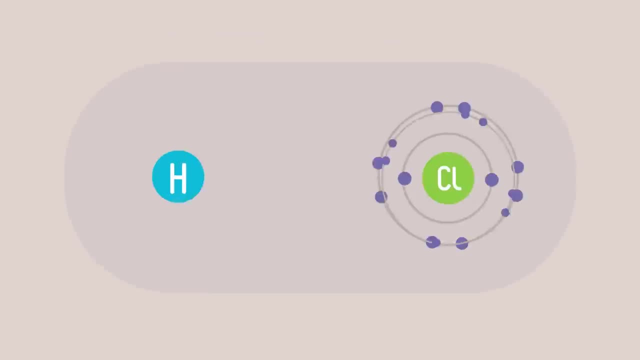 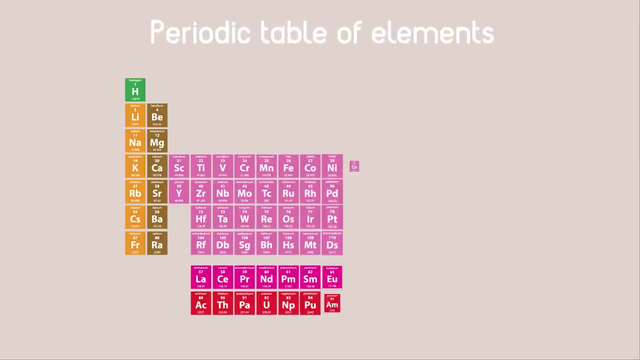 than metallic elements with nearly empty shells. We also see why atoms bond If there is a space in their outer shells. electrons from other atoms can be attracted in by this effective nuclear charge, but only until the shell is full. So let's start with the periodic table of elements, omitting the noble gases. 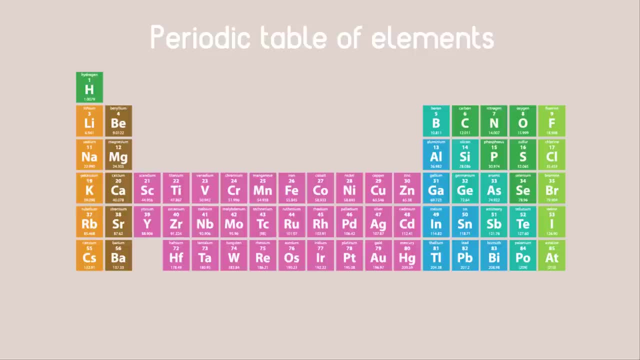 And this last row of radioactive elements from our periodic table. Note that hydrogen, with its half-filled shell of electrons, heads up group four, as well as being in group one with its one outer electron, and group seven with one electron missing. 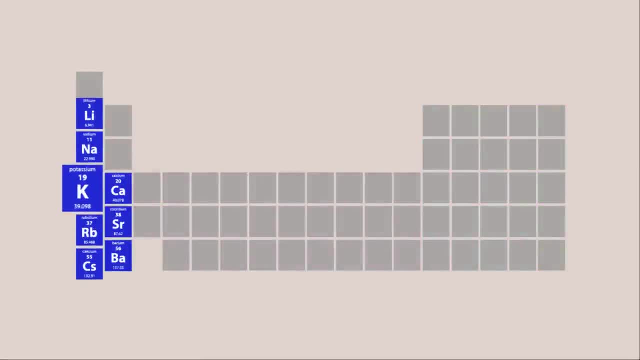 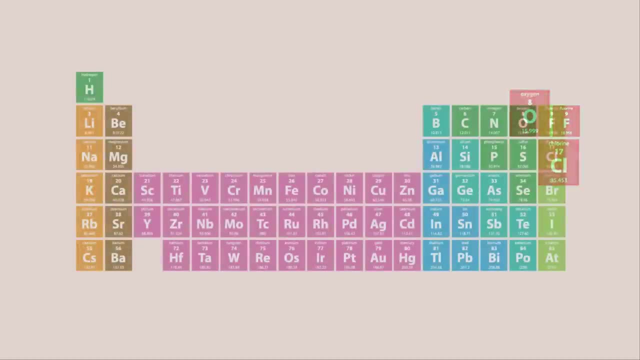 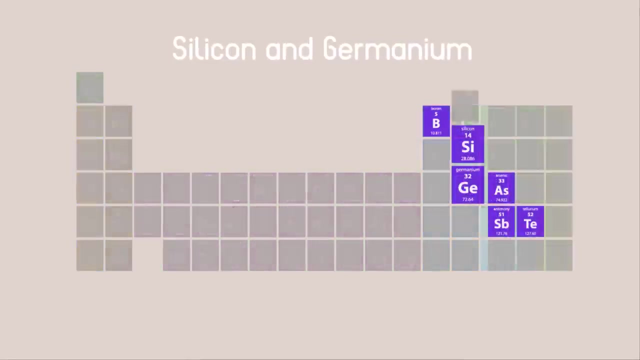 Here are all the very reactive metals like potassium. Here are all the very reactive non-metals like oxygen and chlorine. In between, the elements gradually change from being metallic to non-metallic, with some like silicon and germanium. neither one nor the other. 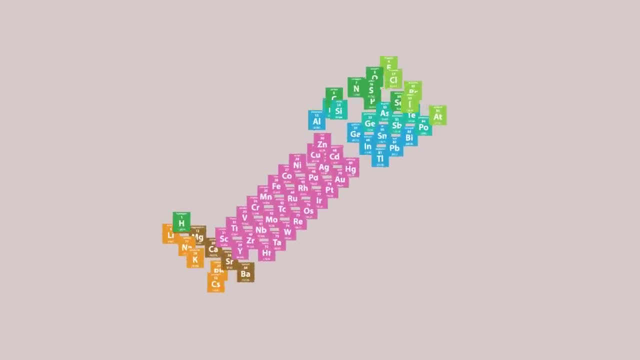 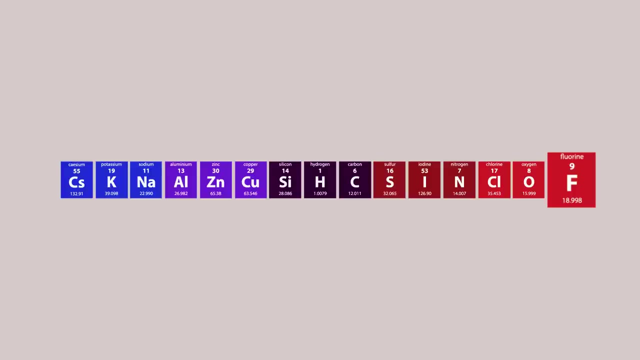 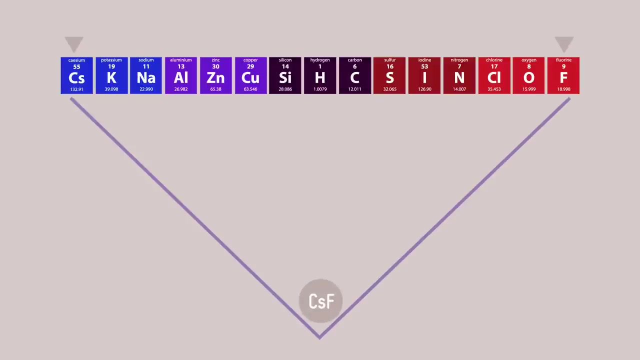 If we twist the periodic table clockwise and then squash it flat, we pretty much have the elements arranged from the most metallic caesium to the most non-metallic fluorine. When these two extreme elements react, they form the stable white salt caesium fluoride. 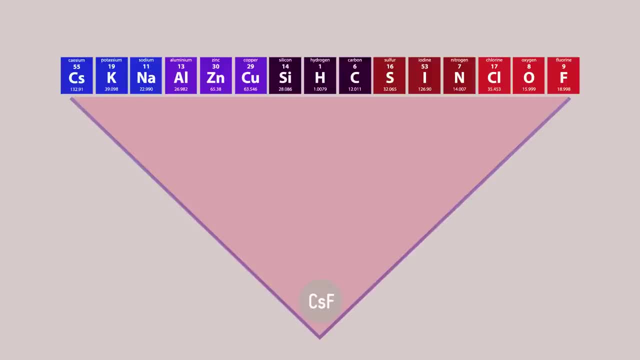 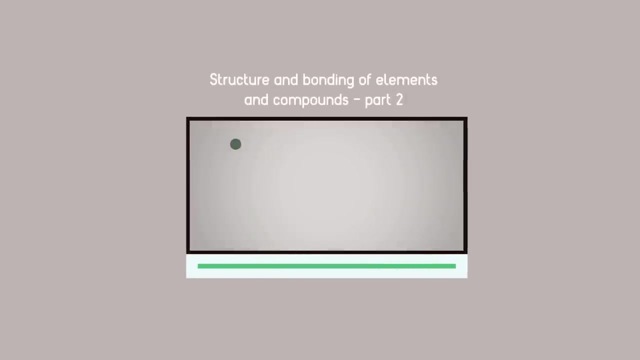 We now have a triangular space where all other combinations of elements can be situated. Elements are along the top and the space will be filled with compounds like brass, sulphur dioxide, sand and salt. By considering the reaction between pairs of elements like this, we will show in part: 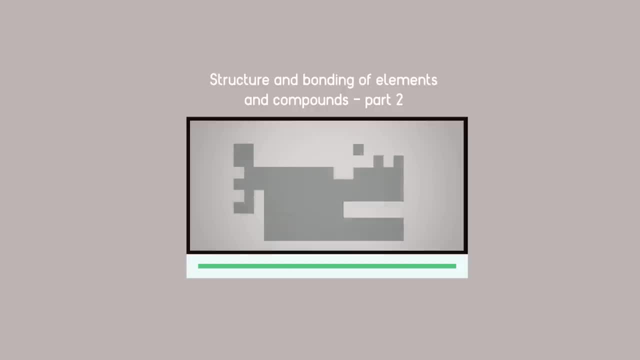 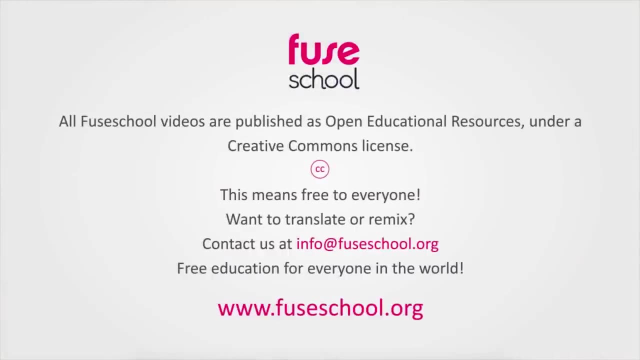 two of this video that there are only four types of bonding possible. We have two types of bondings: one is non-metallic with a non-metallic sulfuride and one is non-metallic with a non-metallic sulfuride, and those have to be completely different. than the other two. Remember, this is just a mummy. there is no next time between the two, but I do want to mention some. This is the nuestra. I know it sounds pretty crazy to say this, but you can actually do. things with a normal human, See you.